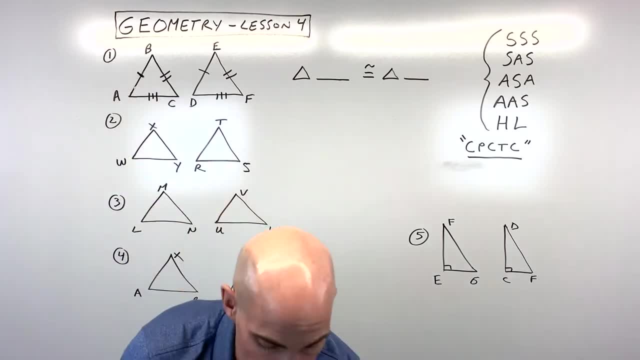 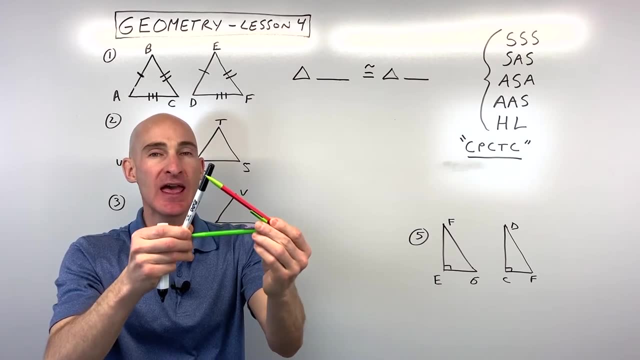 place it on this one, it's going to be an exact match. It's kind of like this: if I were to take three different side lengths, like say, for example, these three pencils and three markers here, if I were to like disassemble this triangle, okay, mix all these sides up, construct them in another. 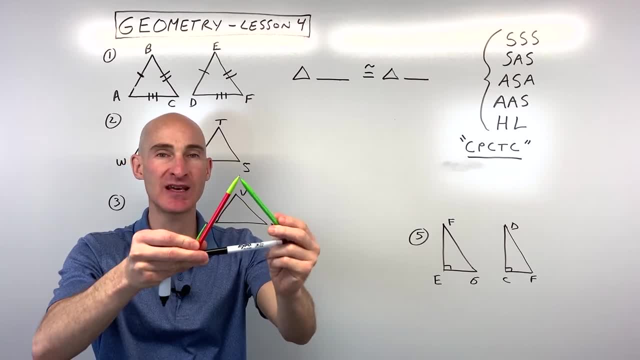 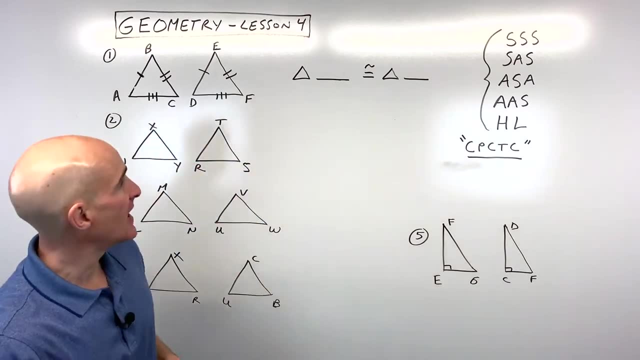 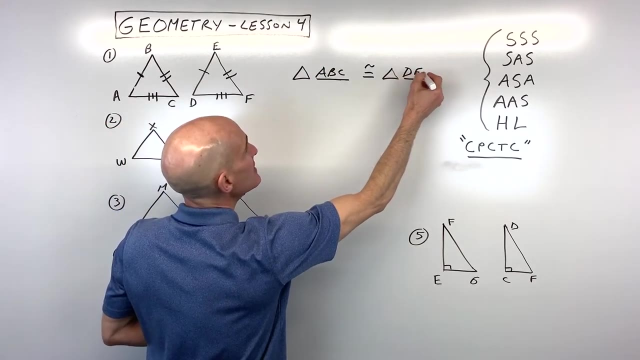 manner okay, such that they're end to end, vertex to vertex, endpoint to endpoint. these two triangles that I constructed would be exactly the same. Try it for yourself and you'll see. So what that tells us, then, is that we can say: triangle ABC is congruent to triangle DEF, and the key thing, when. 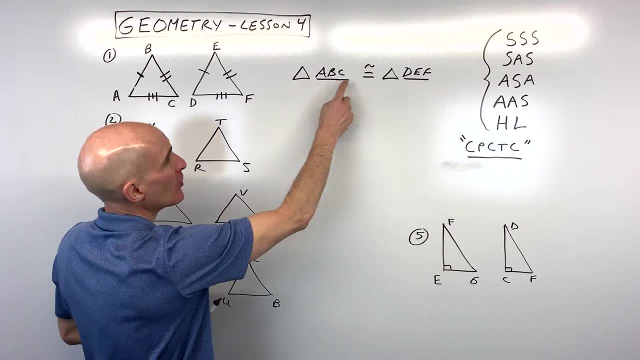 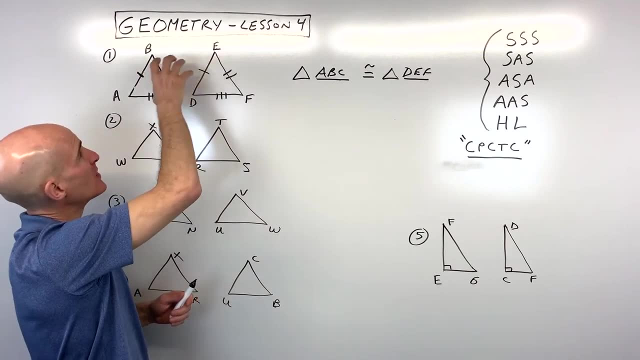 you write, this triangle congruence statement is that angle A matches up with angle D and then B matches with angle E and C matches with angle F. You don't want to have it set up such a way, when somebody matches up those corresponding vertices, that they don't match up, that they're not. 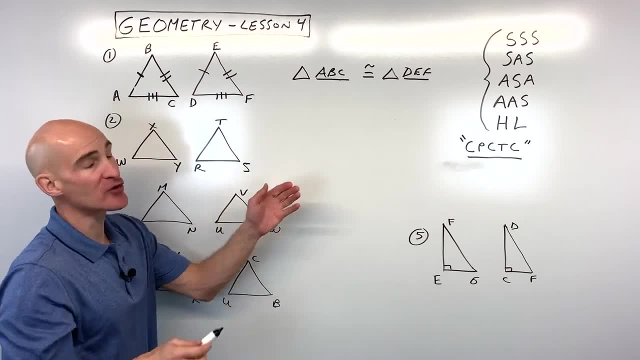 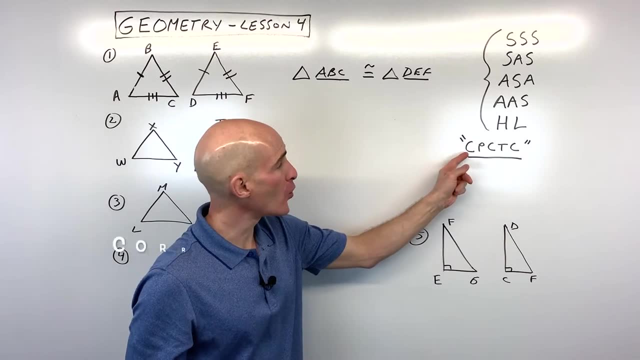 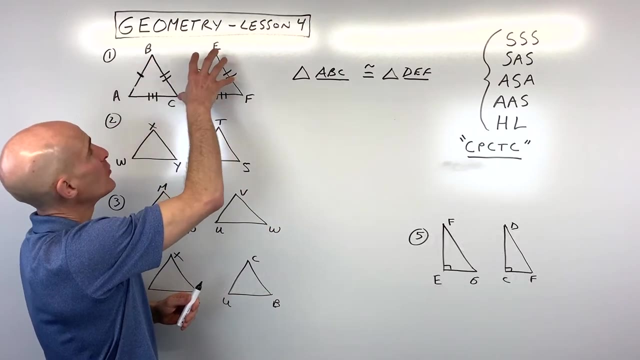 congruent. So once you get to this point where you prove the triangle's congruent, we can use something that's referred to as the acronym CPCTC. What that means is: the corresponding parts of congruent triangles are congruent. So what that means is again, if I pick up this triangle place, 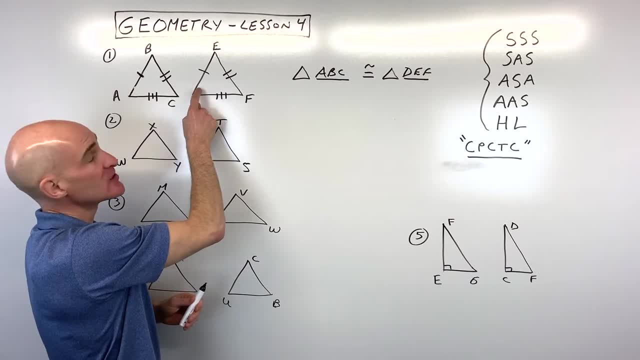 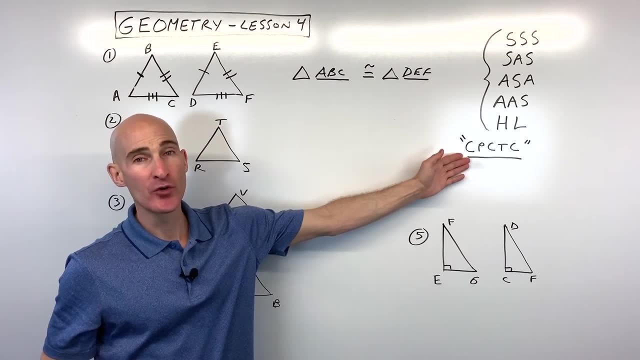 it on this triangle. I'll now know that angle A is congruent to angle D and angle B is congruent to angle E and angle C is congruent to angle F, because once we prove the triangles are congruent, all the components that match up will be congruent. Okay, let's go to the next one side, angle side. 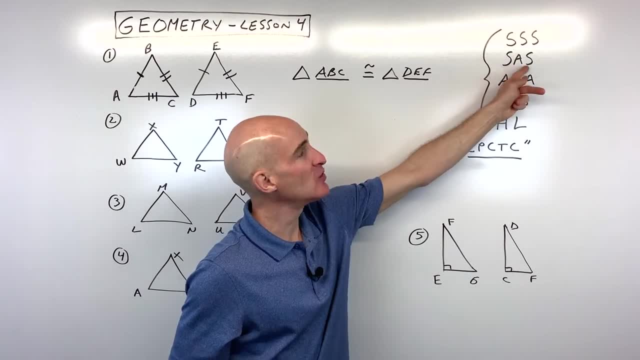 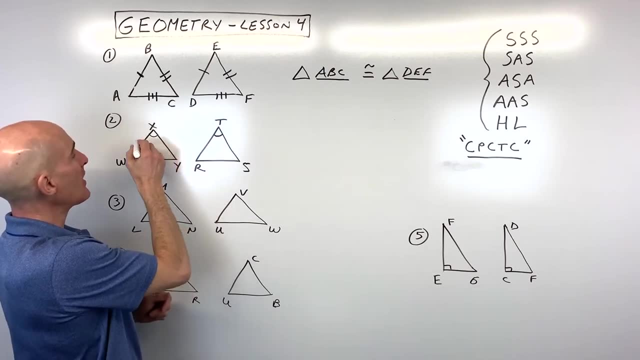 SAS. Now you see how this is written, See how the A is in between the two S's. That means that the angle- say for example here angle X and angle T- that angle has to be in between the two sides that we know that are congruent. So that's what we say: side, angle, side. 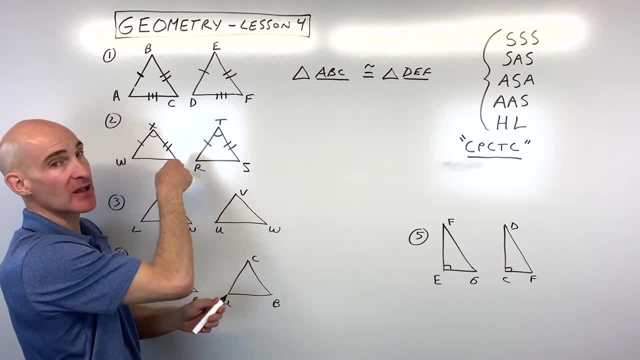 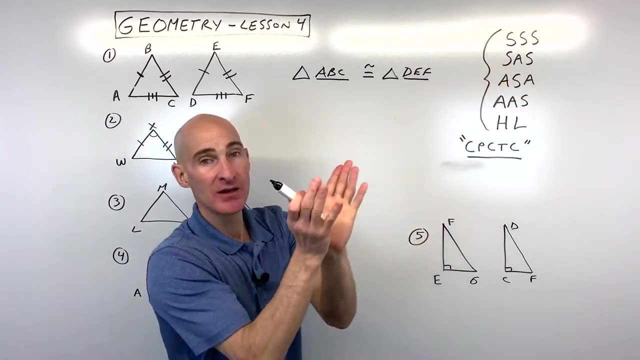 So when you're doing this, you want to think about going around the triangle either in a clockwise or a counterclockwise direction, in order. But this one's pretty easy to remember. just remember it's the angle that's in between the two sides. So here, if we wanted to, 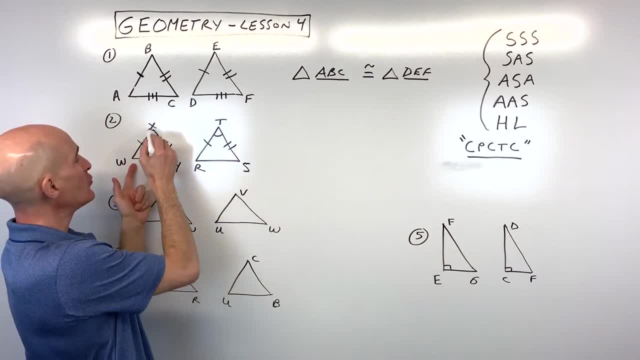 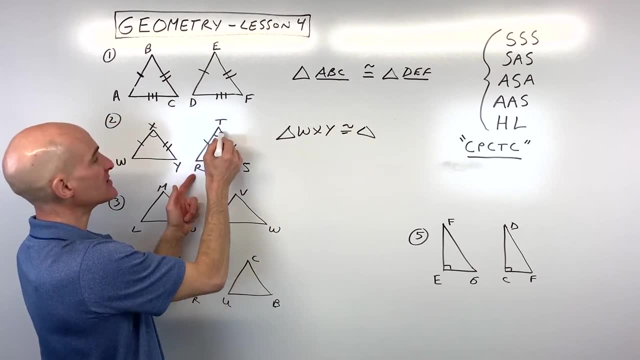 do a triangle congruence statement. we would say: triangle W, X, Y. Okay, so let's write that down: Triangle W X, Y is congruent to triangle R, T, S, R, T, S. Now say, for example: somebody gave us: 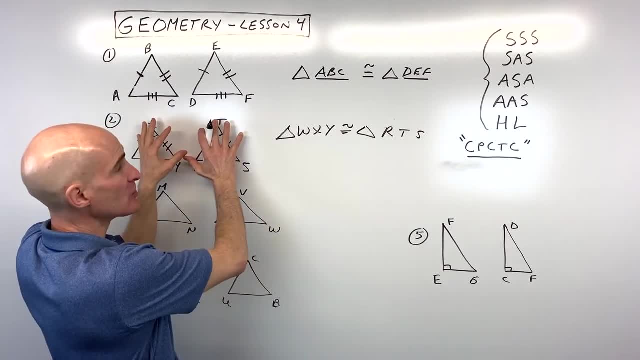 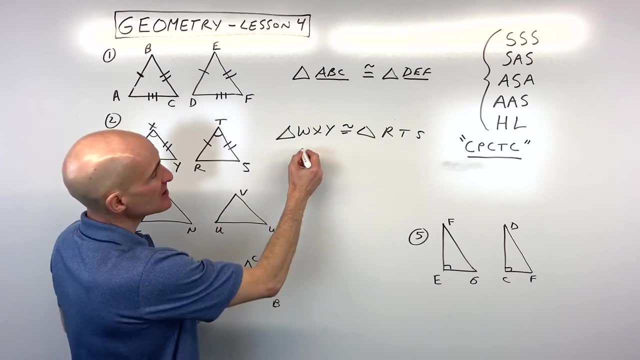 this triangle congruence statement, but they didn't give us the two triangles. Well, we could go ahead and draw the two triangles and then make sure that we have the corresponding vertices matching up, But say, for example, somebody says to you: uh, Mario, what segment is congruent to the triangle? 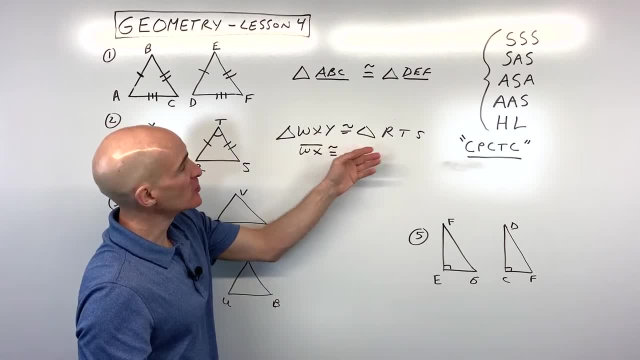 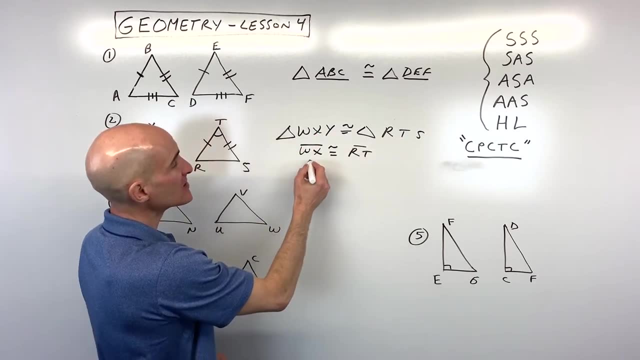 What's congruent to W- X? Well, just by looking at the triangle congruence statement I can see the first and second. see W and X will match up with first and second. R, T, right, Or I could say angle Y is congruent to. 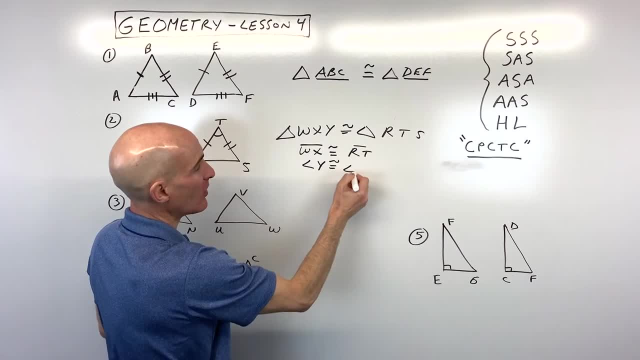 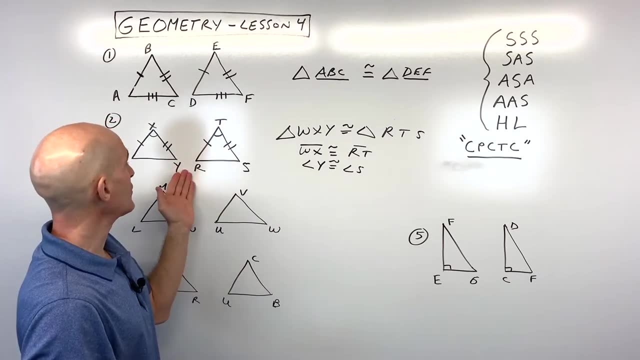 see how. that's the third. This is going to match up with the third angle S. So with the triangle congruence statement. without even seeing the triangles, we'll know what components are congruent. But this is the side angle side. Let's go to the next one angle, side angle. So here you can see. 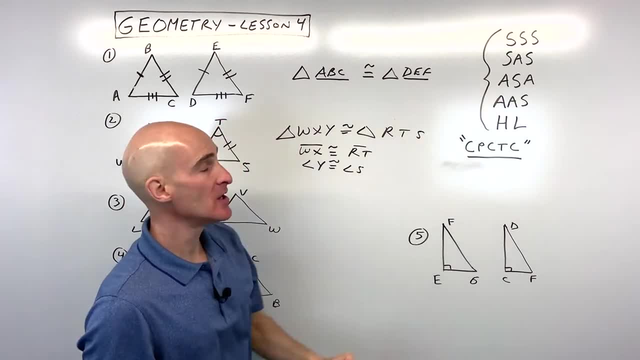 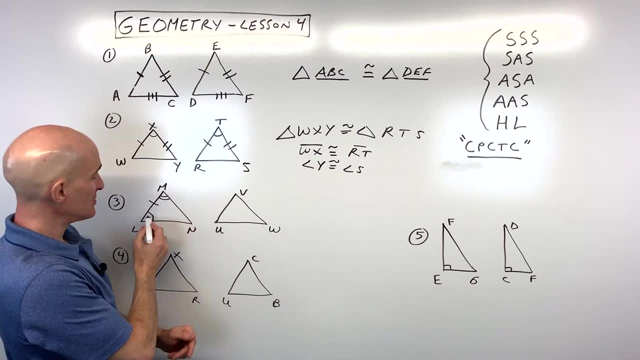 that the side is in between the two sides. So if you look at the triangle congruence statement, it's in between the two angles. So what that would look like is angle side, angle. Now notice how I put two different marks just to differentiate these two angles. These angles are not necessarily congruent. 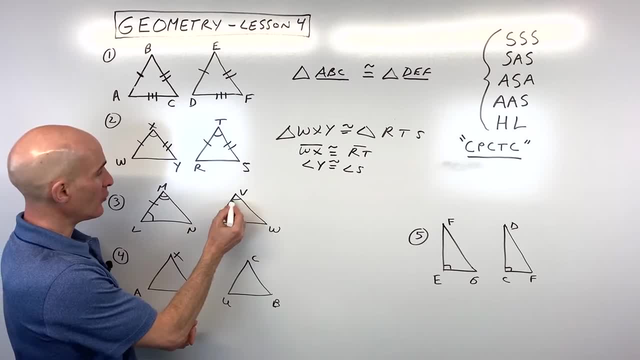 right. And then here we have angle U, angle V, but it's the side that's in between those two angles. as I go around the triangle, either clockwise or counterclockwise, It's what they call the included side, meaning in between. Over here this is called the included angle. So here we have. 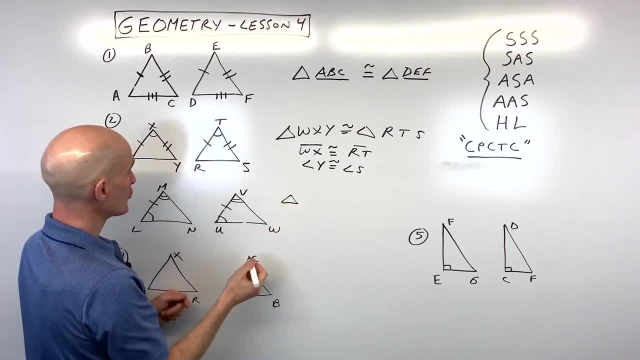 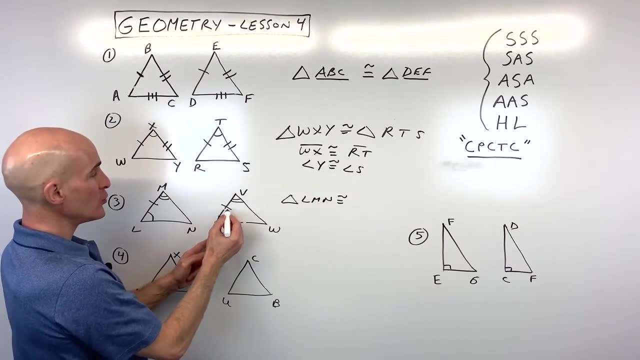 angle side angle. angle side angle. Again, if we want to write our triangle congruence statement, we'd say: triangle L, M, N. L M N is congruent to U, V, W And if you have any, you know. question. 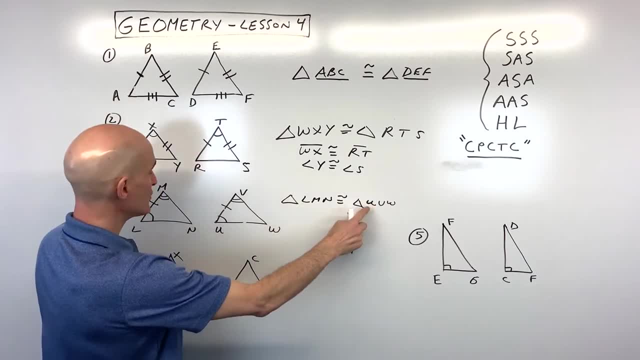 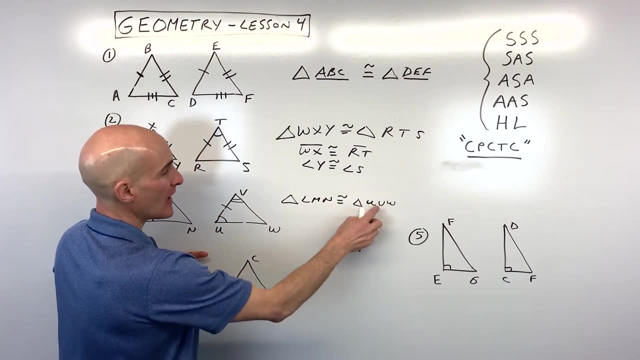 did you write it correctly? Just go back and say: well, is angle L congruent to angle U? Okay, yep, it looks like they're the same. Is angle M congruent to angle V? Okay, yeah, they're the same. And then is angle N congruent to angle W? Yeah, these would be the same as well. 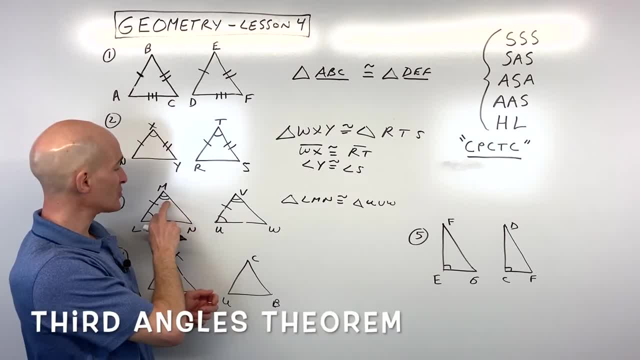 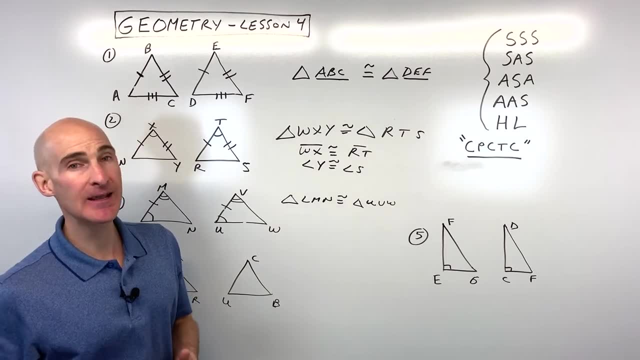 And we know that by the third angles theorem, meaning if two angles in one triangle are congruent to two angles in another triangle, automatically the third angles are going to be congruent as well, because all those angles have to add up to 180. And that's how you know that these are going to be the same. Okay, for. 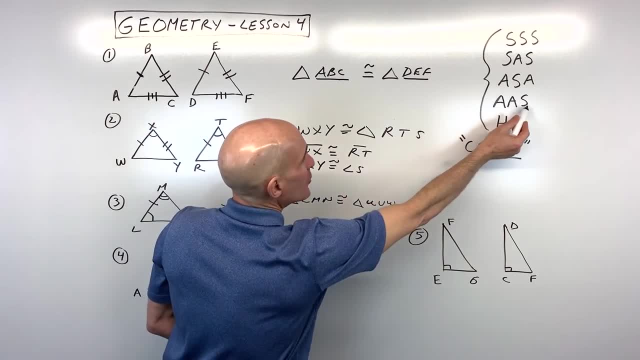 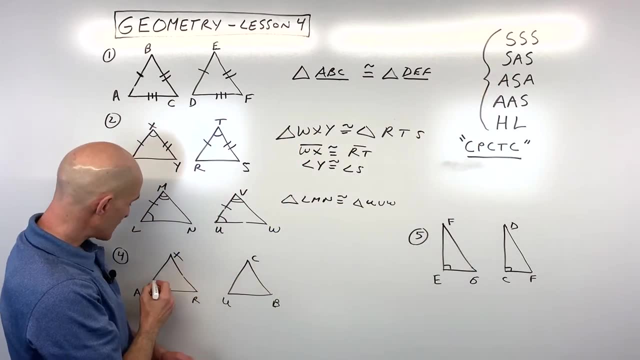 number four, we're going to look at this one angle angle side. This one tends to be a little bit tougher for students because it's not so easy as the first three. Angle angle side would look something like this: Angle A, angle X and then this side here, XR. I could also do it like this: 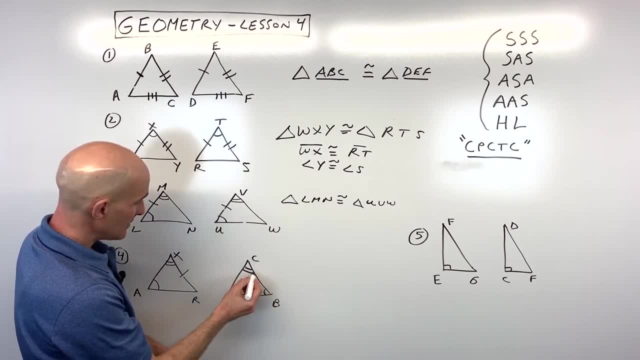 I'll say angle B, angle C and then angle side. I'm sorry, side CU, But the key thing is see, here I'm going like angle, angle side. I'm going around like clockwise, right, Here I'm going counterclockwise. 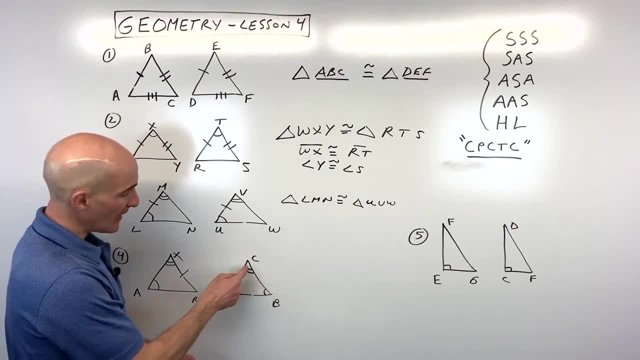 angle angle side. But you want to go in order. You don't want to go angle angle, skip that side, go to this side, right. So you want to make sure you're doing it in order. Now how would you write? 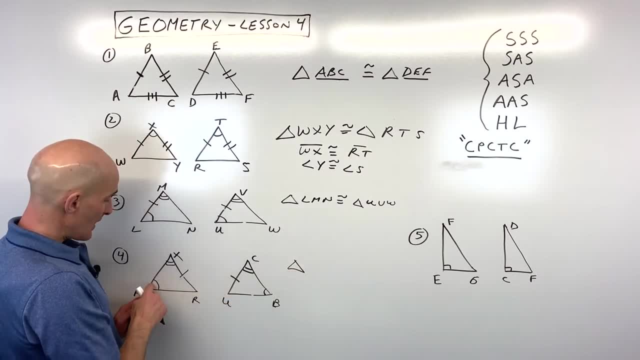 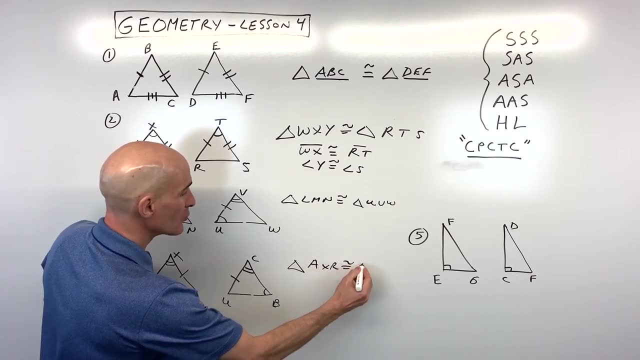 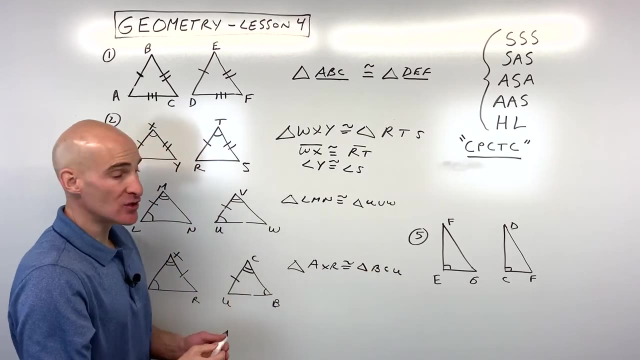 the triangle congruent statement for this one. Well, let's do angle angle side. So I'm going to go. triangle AXR is congruent to triangle BCU. Now, if you want to play around with this, you can draw. 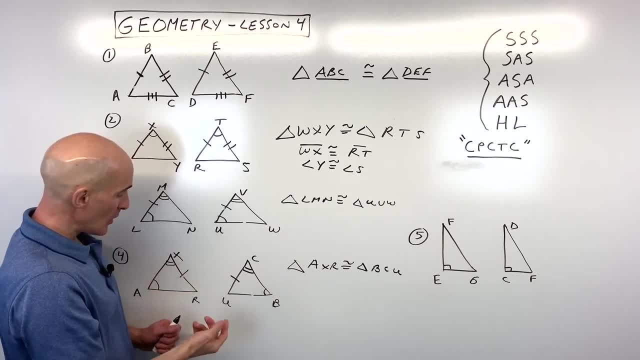 these on a sheet of paper. Go ahead and cut this one out, cut this one out, And when you match them, what you're going to see is- this is actually like a reflection, Like if I was to take this and like flip it or fold it. then you can see that B and A match up, C and X match up, and then U and R would. 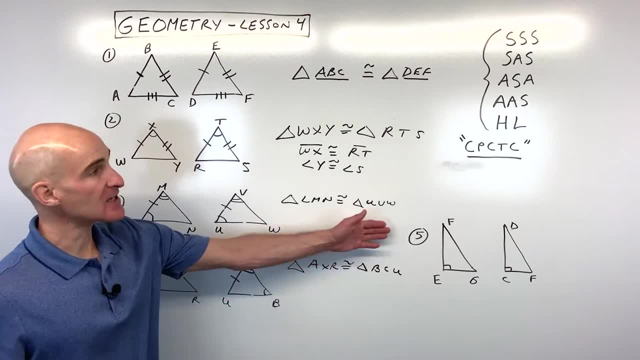 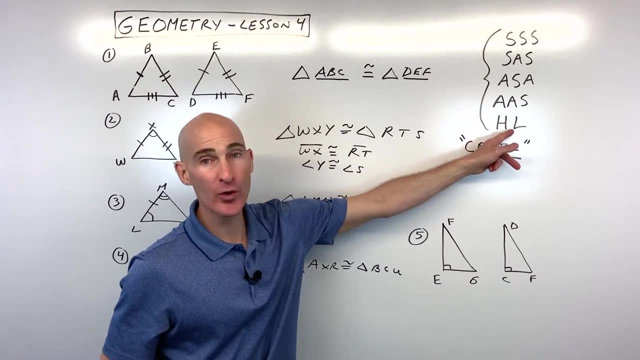 match up And you can see that here in the triangle congruent statement. Last one: this tends to also be one that's called the hypotenuse leg. okay, triangle congruence theorem, And this one only works when you have a right triangle, meaning you have that right angle. So a lot of times, students, 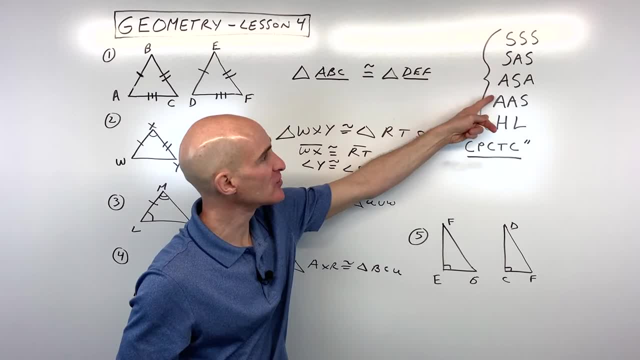 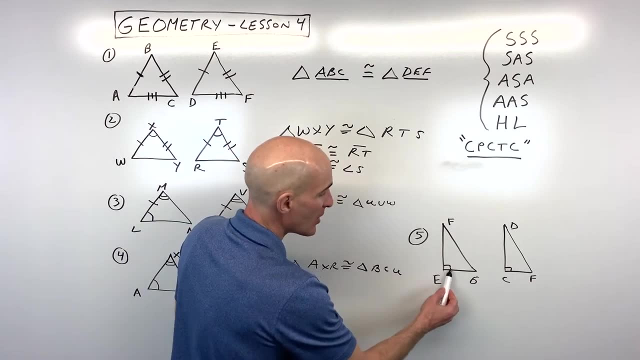 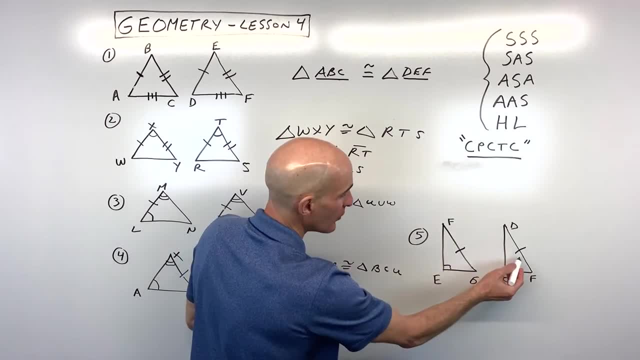 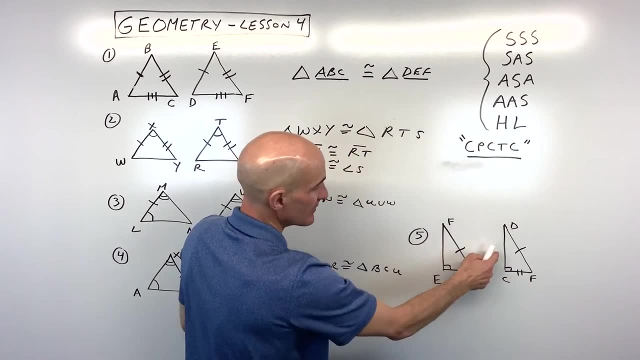 are congruent, okay, So that's the side that's across from the right angle, And then one of the right triangles is congruent. For example, this leg and this leg are congruent. or we could say: this leg and this leg are congruent. Just because it's a right triangle doesn't mean it has to be a. 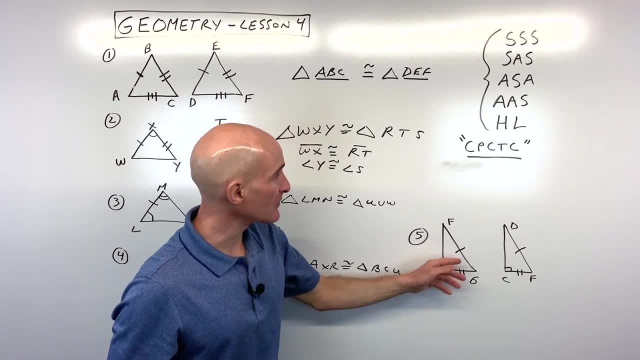 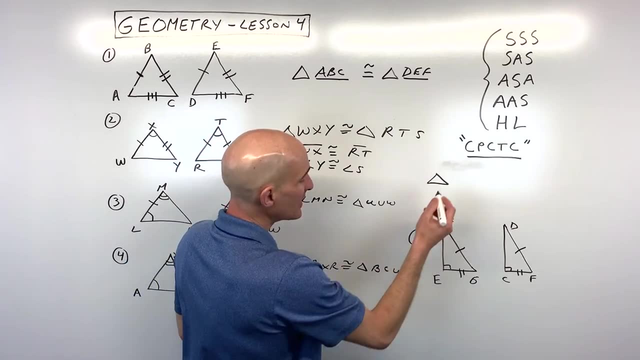 hypotenuse leg. It's just that when you have a hypotenuse leg, this will only be applicable to when you have a right triangle. So for this one let's write the triangle congruent statement. And then I want to get into some examples showing you how to show triangles are congruent. So here we've. 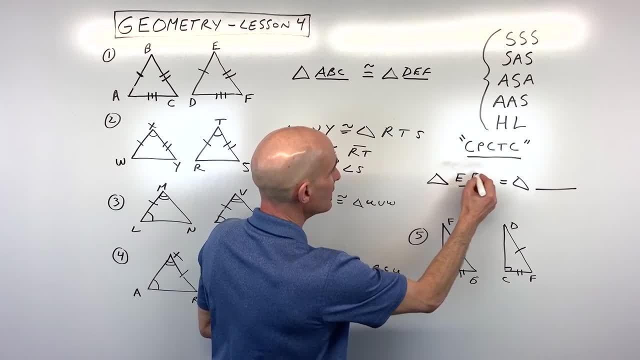 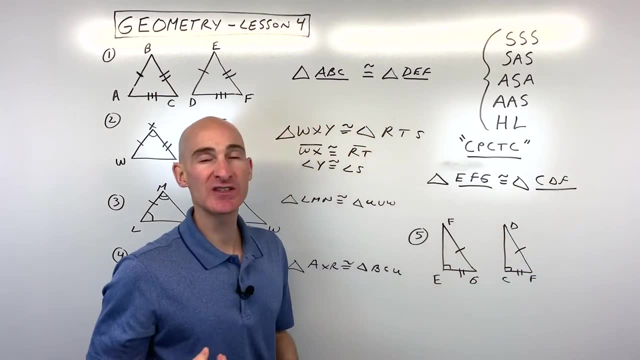 got triangle EFG. EFG is congruent. And then I want to show you how to show triangles are congruent. So triangle CDF And you got it. So let's do some examples. Number six: see if you can do these on. 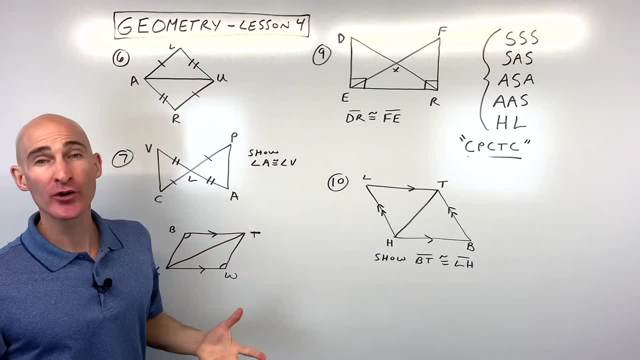 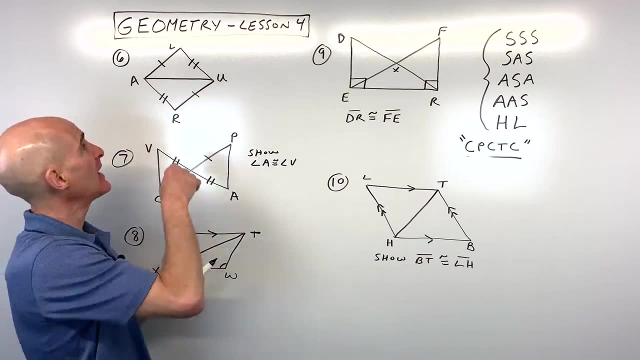 your own. How would you prove these two triangles are congruent or how would you show that they're congruent? Well, when I look at this, the first thing that I notice is that there's two triangles here, And you see how the top triangle and the bottom triangle see how they're sharing the side. 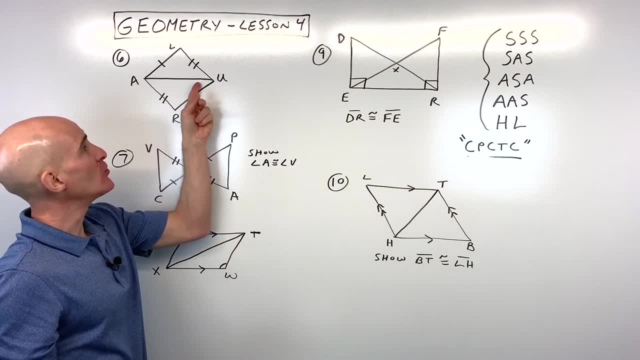 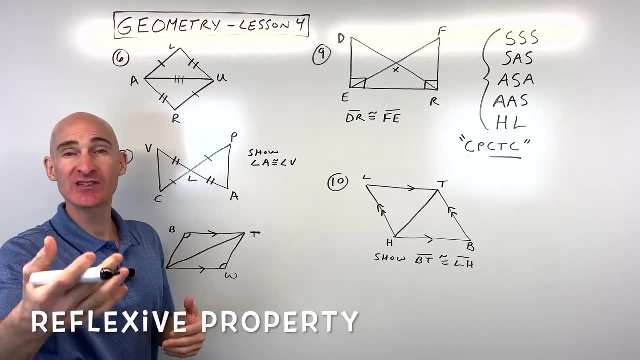 right here: AU. So what we could say is we could say that AU is congruent to AU by the reflexive property. Reflexive, it's just like a reflexive property. It's just like a reflexive property. Reflection, like: if you look in a mirror, you're the same height in the mirror as you are in real. 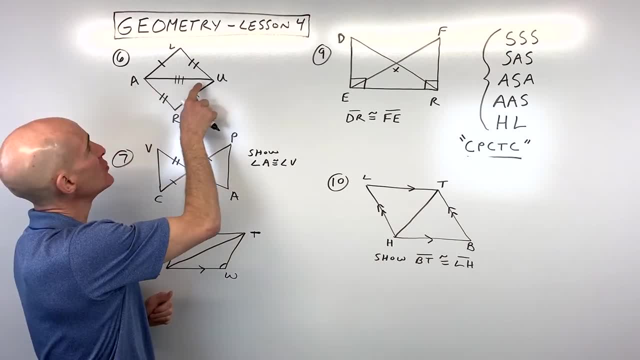 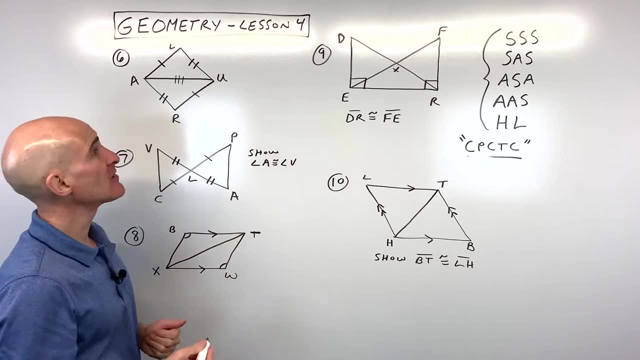 life. They're the same right. So AU is congruent to AU. Now look what we have. We have three sides in the top triangle are congruent to three sides. in the bottom triangle We can say that the triangles are congruent by the side side side. See three sides congruent to three sides. 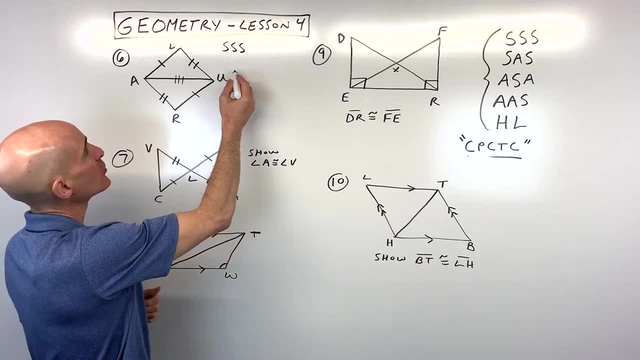 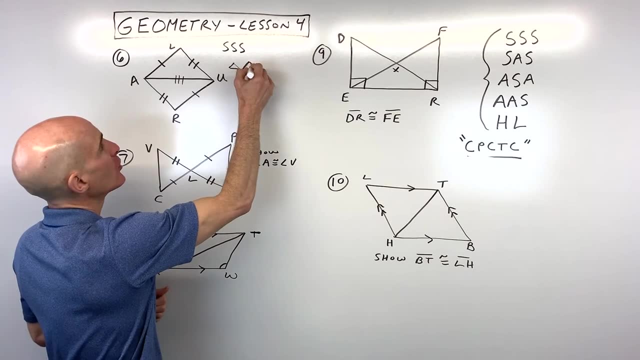 Triangle congruence theorem. Now, if you want to write the triangle congruence statement, what I would do is I would say: triangle ALU. Okay, now look at my strategy here. Sometimes students have a challenge with this, and you might. 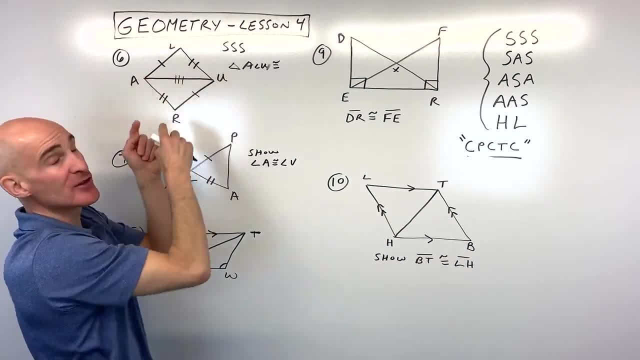 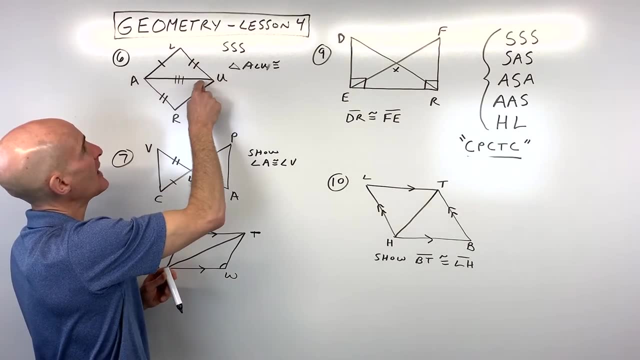 as well. What you want to do is you want to figure out a way to go around this triangle that makes sense to you. So, for example, I see that there's one marking here, two here, three here. So if I go around ALU, it's like one, two, three. If I follow that same pattern with this triangle. 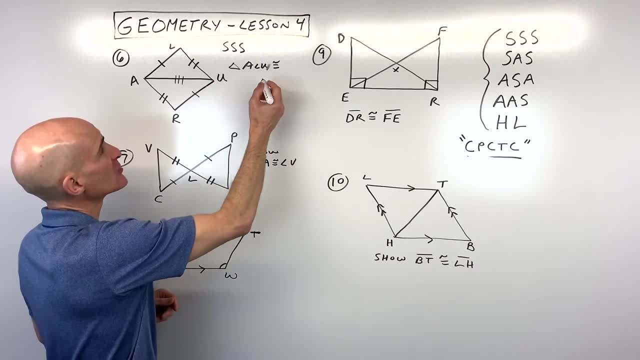 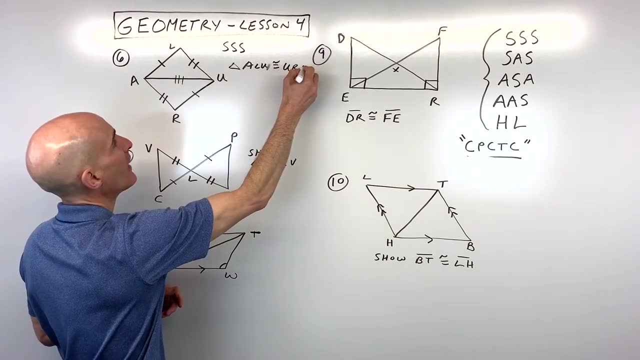 one, two, three. right, I know the sides are going to match up and the angles are going to match up, So this is a triangle URA. back to U. So U R A triangle URA. Okay, let's go to number seven now. Number seven: this one's a little bit. 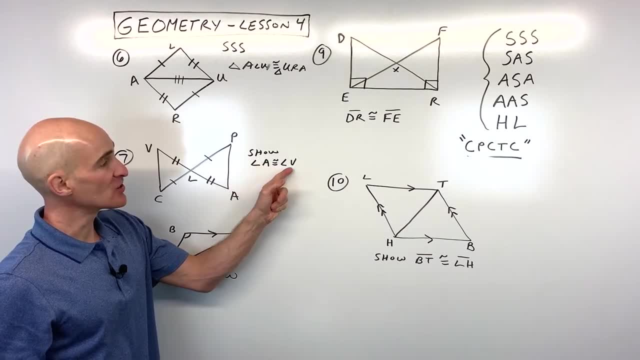 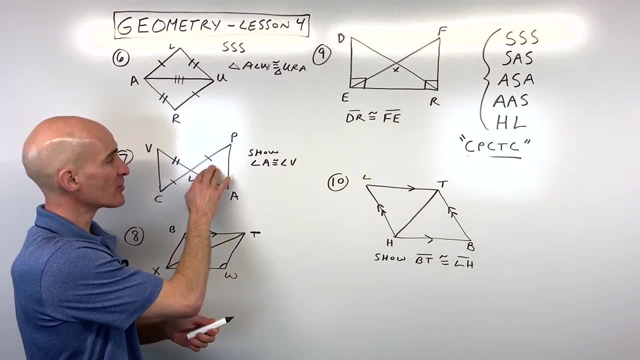 different problem. What I want you to do here is show that angle A is congruent to angle V, So this angle is congruent to this angle. Now, before we get to that, though, it's helpful to show that these two triangles are congruent. Once we know that they're congruent by the CPCTC. 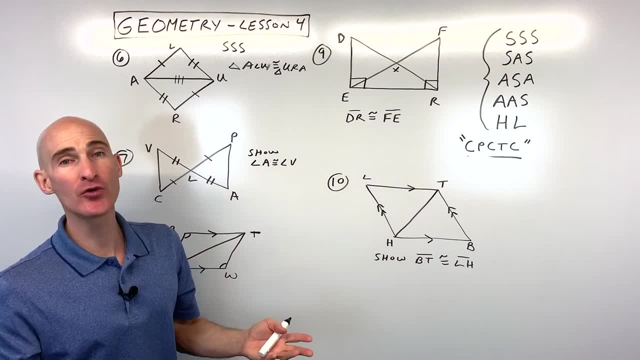 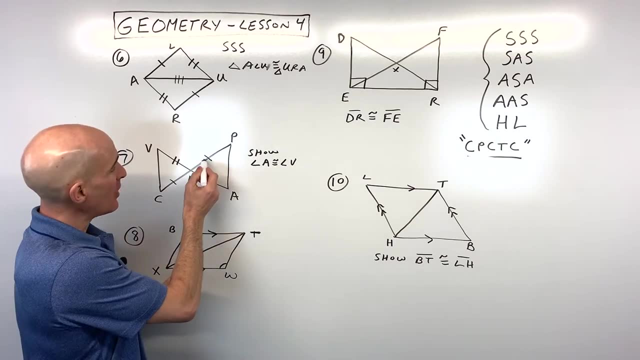 we know that the corresponding parts, or the parts that match up, will also be congruent. So the question is now is how would you show that these two triangles are congruent? Well, what you might notice is that see how this forms like an X. see these two line segments. 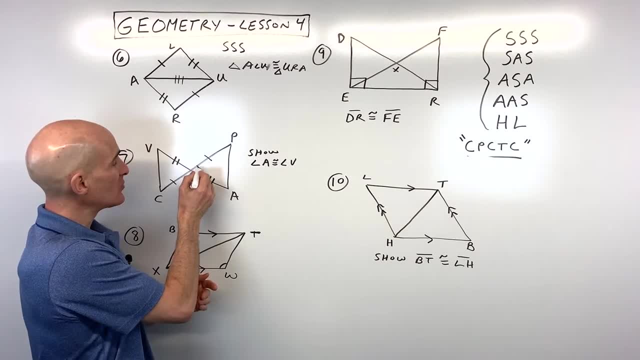 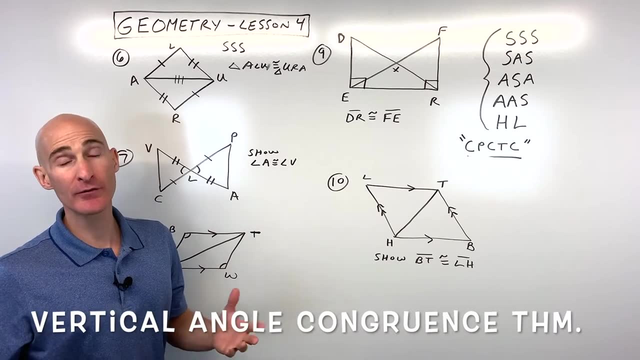 see how they cross right here at point L. We know that these angles that are across from each other, these are vertical angles, And we know that vertical angles are congruent by the vertical angle congruence theorem. So now look what we have. We've got side angle side. See how the 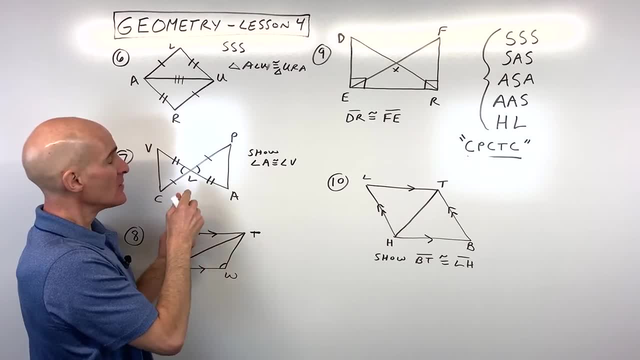 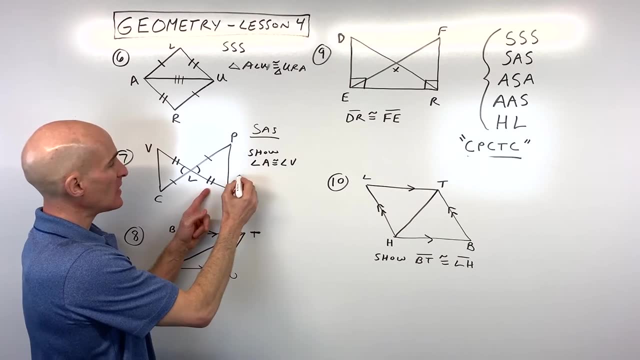 angle is in between these two sides And over here we have side angle side. So we know the triangles are congruent by side angle side. Let's just write that down And let's write our triangle congruence statement. So we have triangle. Now watch my strategy here. 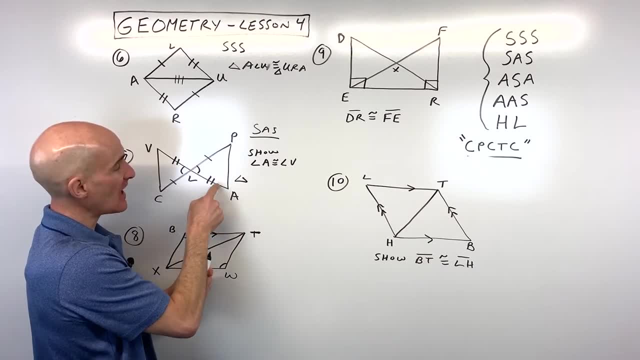 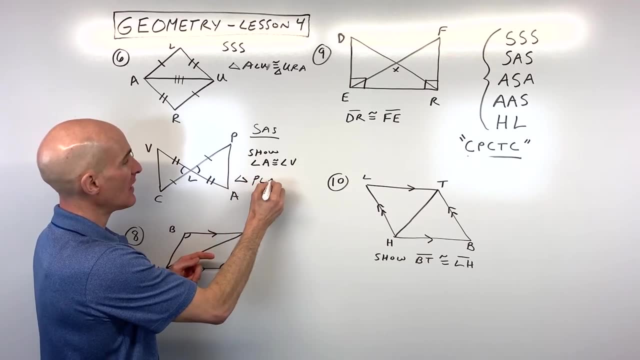 I'm going to go side one angle, side two, So I'm just following the side angle, side pattern, right. So that's going to be triangle, PLA, PLA is congruent to triangle. What did I do? One angle. 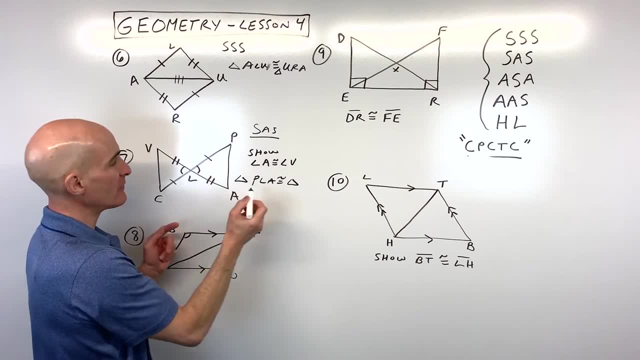 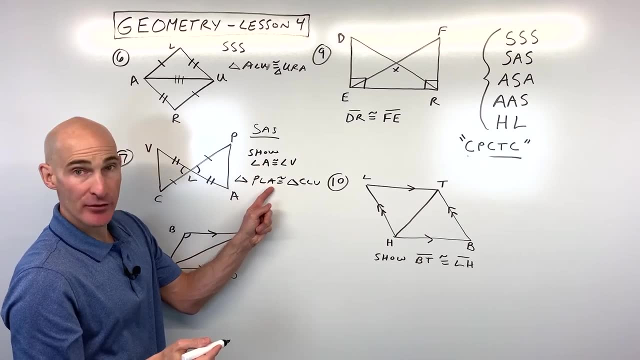 two. So I'm going to do one angle two. So this would be CLV, CLV, And now we have our triangle congruence statement. You can see that angle A- see how it's the third component here- is congruent to angle V, the third one over here. So they see how everything matches up. 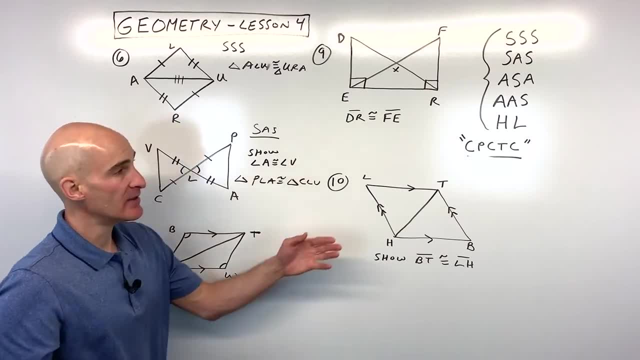 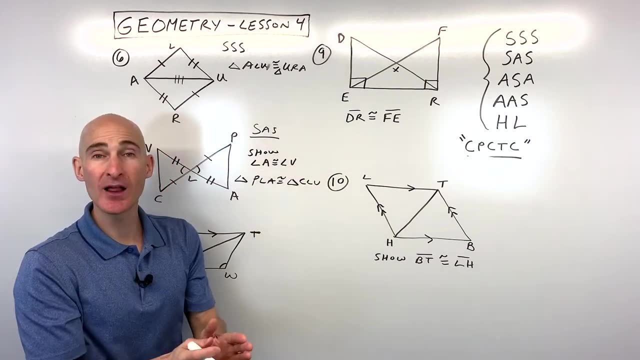 So we could say that angle A is congruent to angle V, and that would be by the CPCTC. Now I'm going to put a link at the end of this video where I go in more depth with two column proofs, what we call. 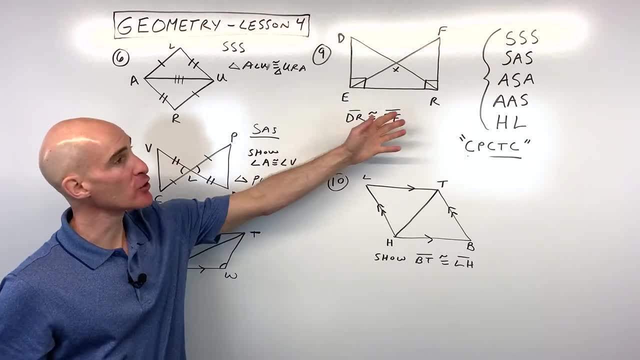 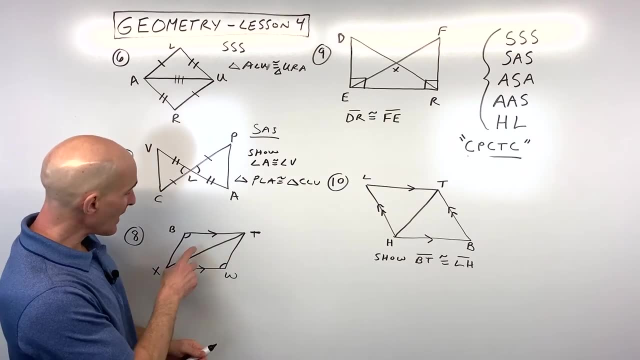 two column geometry proofs Here. we're just getting familiar with working with these five triangle congruence theorems, But I'll show you that at the end of this video. So for number eight, we've got these two triangles here. I just like for you to see if you can prove that these two 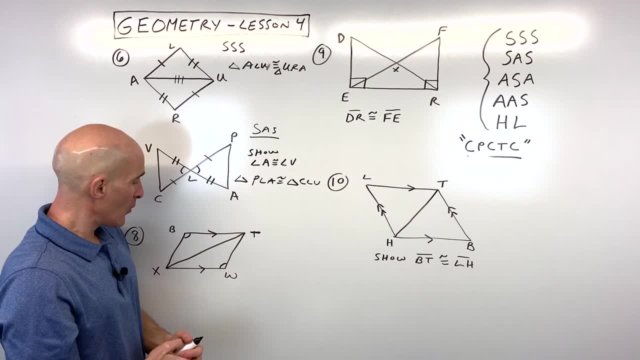 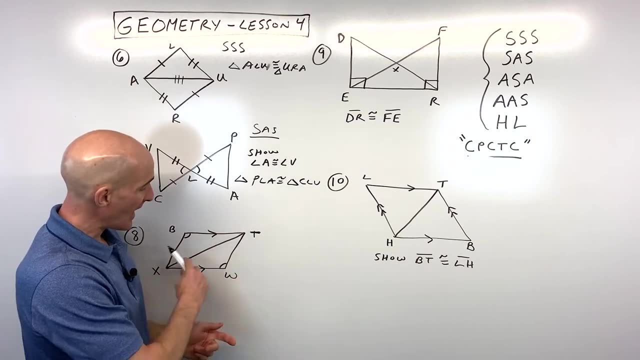 triangles are congruent. Okay, by one of these five methods. Well, what's interesting about this problem is you see these little arrows here. Remember those arrows? tell us what. It tells us: that the lines are parallel. So what I like sometimes like to do is I like to extend those. 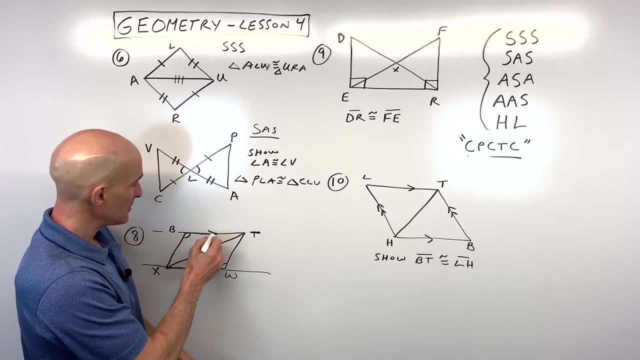 lines. okay, a little bit, just so I kind of you can see it a little bit clearer. And then see this third line here. This is the transversal. See how it cuts across. so what should jump out at you here? so you remember this diagram from a previous lesson. 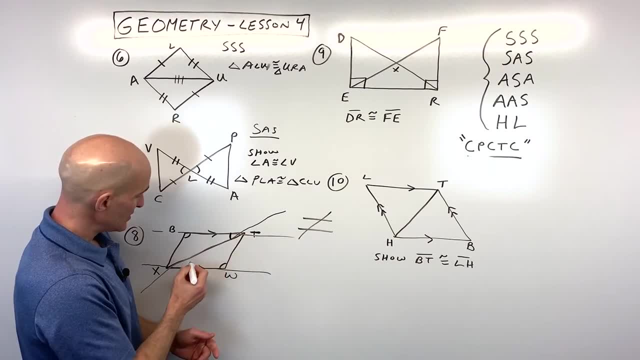 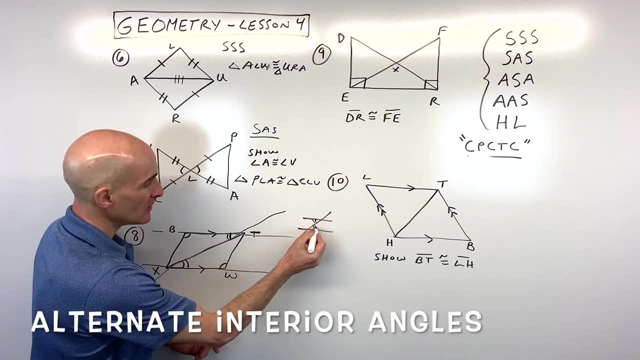 you can see that this angle right here is going to be congruent to this angle right here, by what it's just like: this angle and this angle, those are called the alternate interior angles because they're interior, they're in between the two lines: one's on the left side, one's on the right side. so 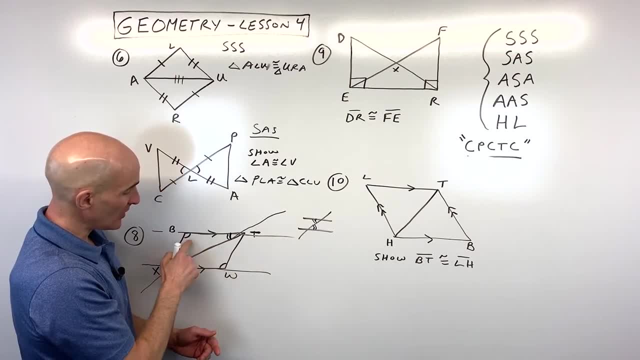 alternate interior angles are congruent. they already told us that angle b and angle w are congruent, and what else do we know is congruent between these two triangles? remember, we need three components. well, you see how they share this side right here, xt is congruent to xt by the reflexive. 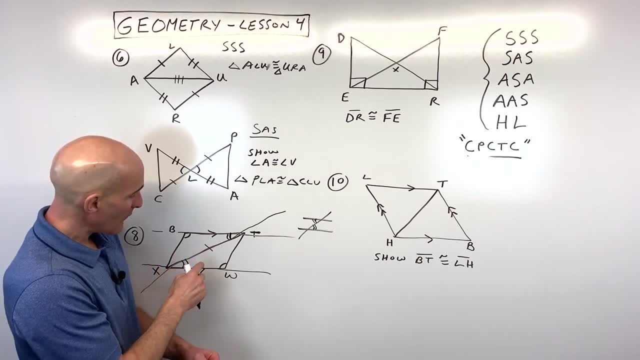 property. let's just mark that there. so now you can see we have what angle, angle side, angle angle side. so if i took this triangle and i rotated it, see, if i picked it up, rotate 180 degrees, everything would, that's congruent, would correspond or match up. so we're going to say this: these 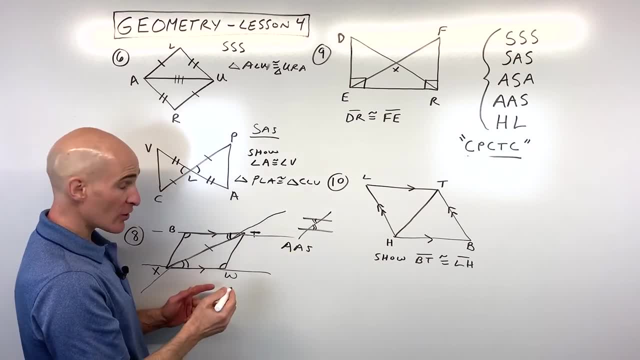 triangles are congruent by the angle angle side. and if we want to write our triangle congruence statement again, you want to be strategic. i'm going to go how that has one mark, two marks and no marks. i'm going to go angled, i'm sorry. triangle. 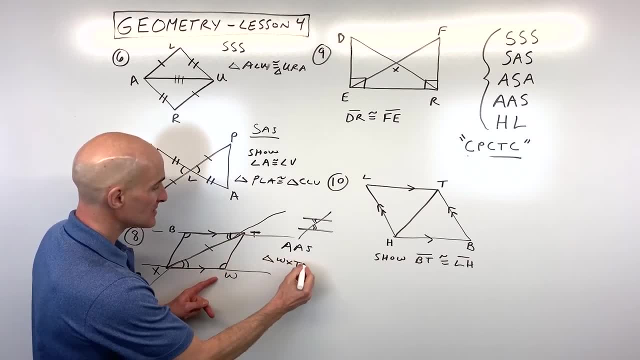 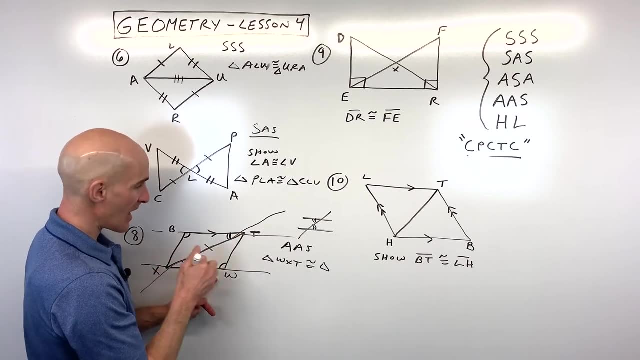 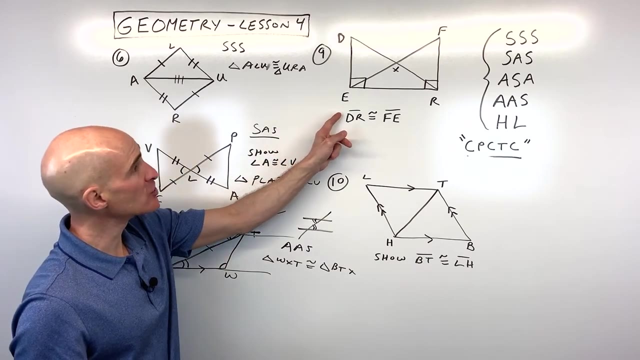 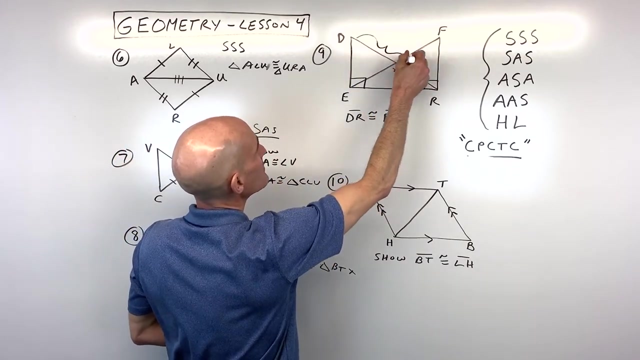 w, xt. triangle w, xt is congruent to triangle c, 120, 120. so b t, x. okay, now let's go to number nine. now, number nine. what we want to do here is we want to show that segment, dr. oh, i'm sorry this one. they tell us that dr is congruent to fe, so let's mark that on the diagram. 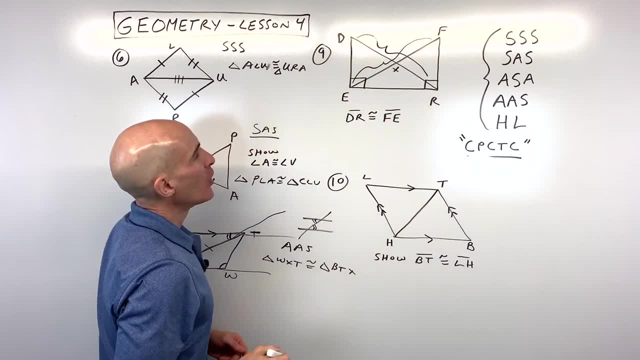 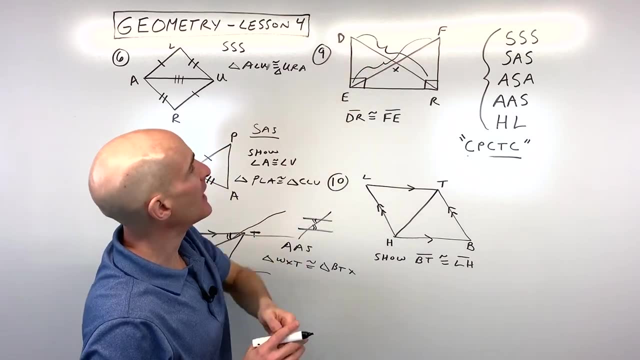 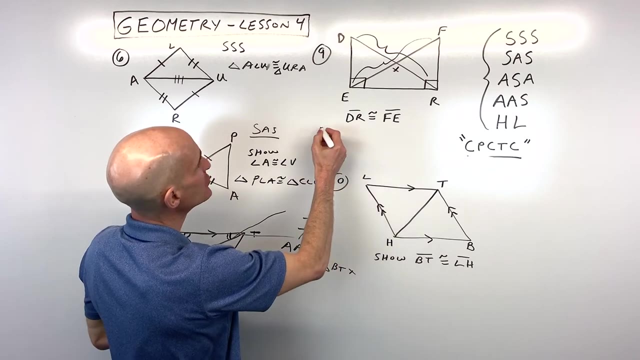 so dr is congruent to fe- okay. so now, what do we know here about these two triangles? we want to show that this triangle is congruent to to this triangle, okay, and what you can do here is- this is a helpful technique- is, when triangles are overlapping like this sometimes, it's helpful to 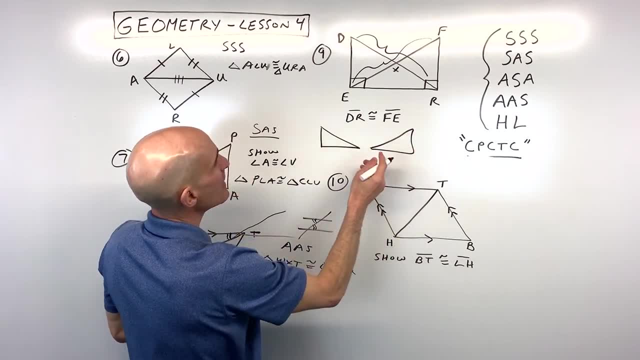 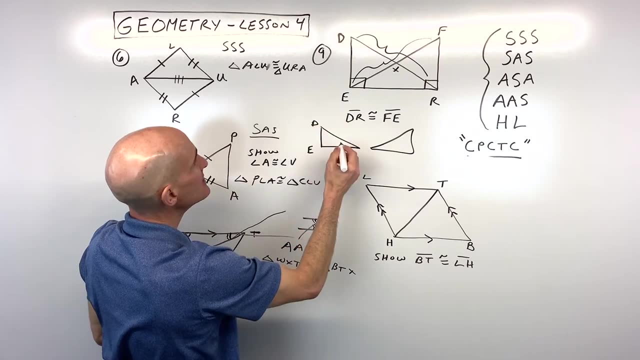 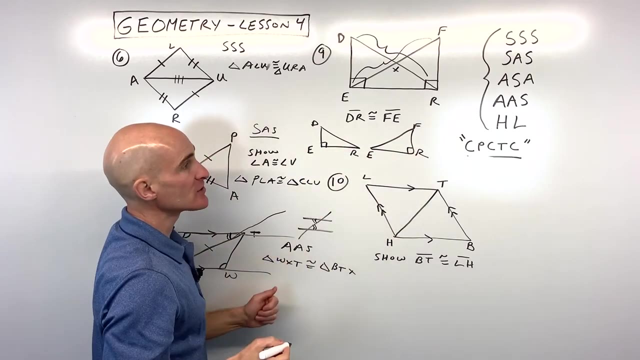 to pull them apart, okay, and draw them separately. so i took this triangle here and this triangle, you can see, this is going to be edr and this is going to be e? f? r. this angle and this angle are right angles. so it might be the hypotenuse leg theorem- not necessarily, but it, you know, could. 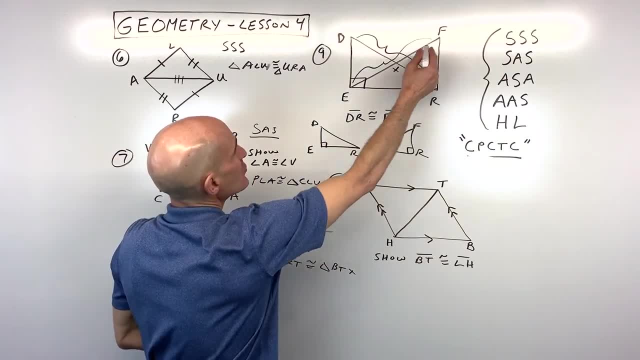 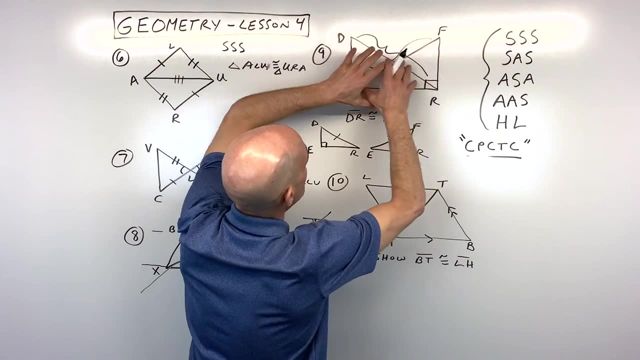 be because they're both right triangles. we know that dr is congruent to ef, so we know that the hypotenuses are the same. and then- this is what's often overlooked- is that see, when i pull these triangles apart, see how originally they both had the same base, the same bottom, this er. so we see. 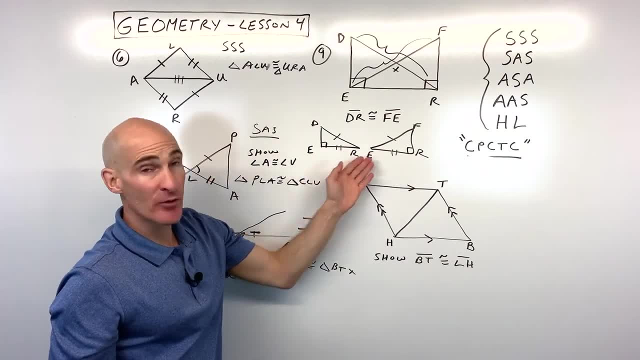 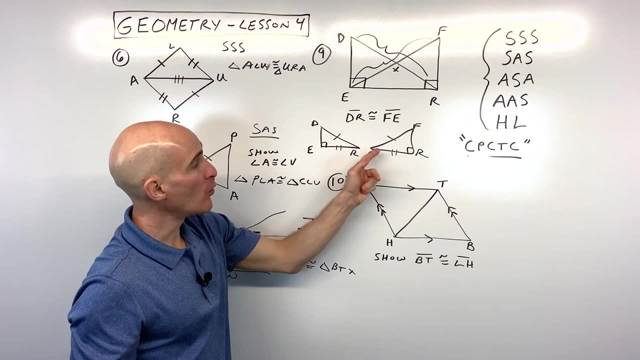 er is congruent to er and that's by the reflexive property, because it was sideways shared. now look what we have. we've got right triangles, the hypotenuse is congruent and one of the legs is congruent, so we know it's the hl congruence theorem. and then we can, you know, say that the 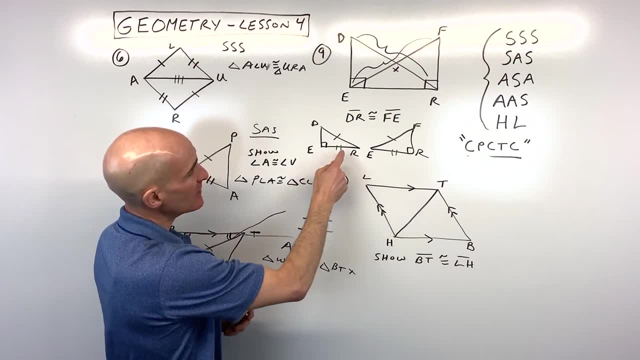 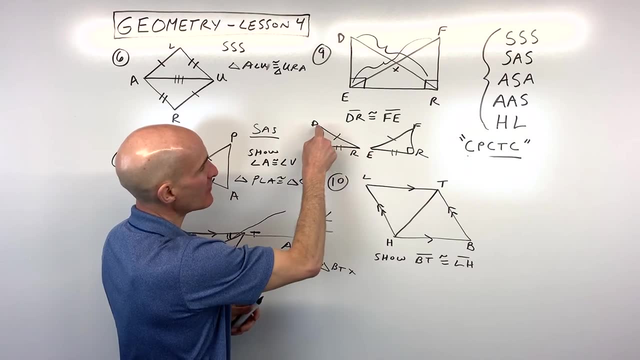 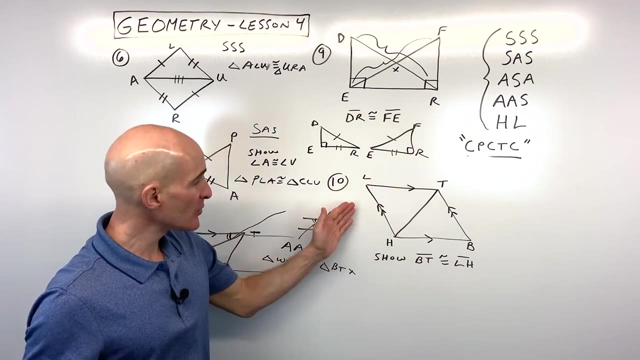 triangles are congruent by hl and then we can write our triangle congruence statement and you can do like dre. okay, now notice i'm doing one, two, zero. basically say on the on the side markings, one, two, zero. i can follow that same pattern: one, two, zero, okay. last example, number 10, here, 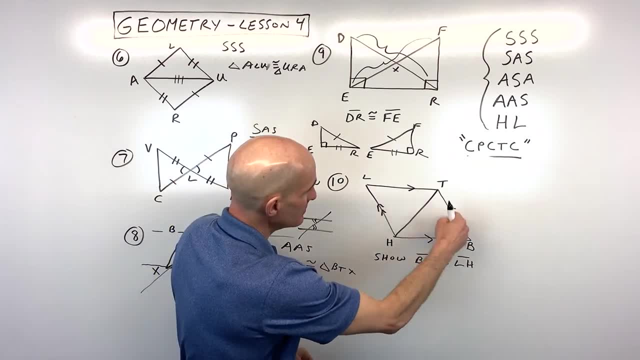 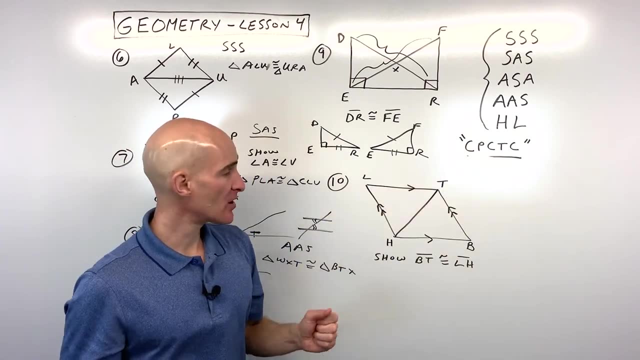 what we want to do is we want to show that segment bt is congruent to segment lh. okay, and we can do that by using the cp ctc. again, the corresponding parts of congruent triangles are congruent, but first we have to show that the triangles are congruent. so how do we show the triangles are? 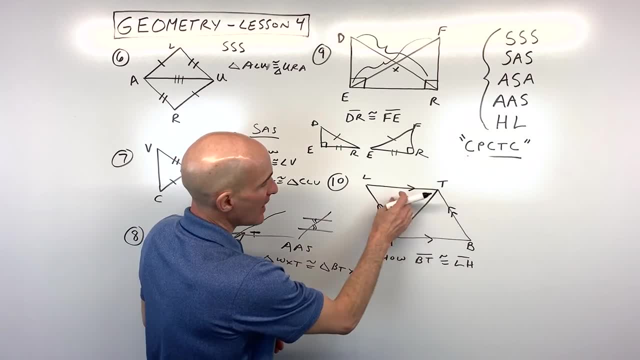 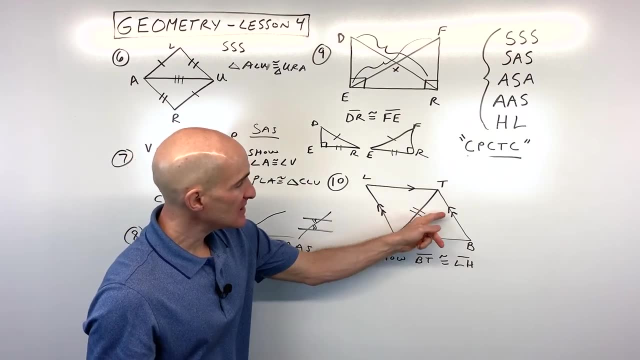 congruent. well, the first thing that jumps out at me is that these two triangles, they're sharing the side ht. so i'm going to say ht is congruent, and then i'm going to say ht is congruent and ht is congruent to ht by the reflexive property, and then we see these double arrows here and 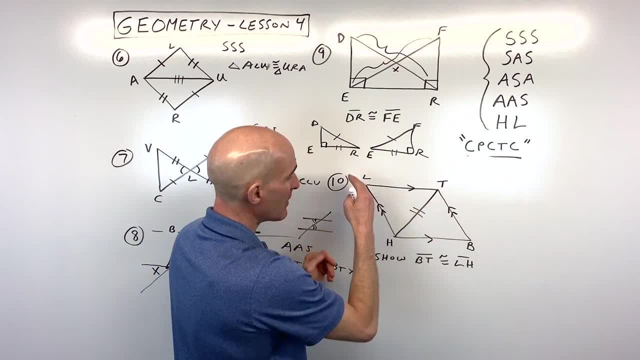 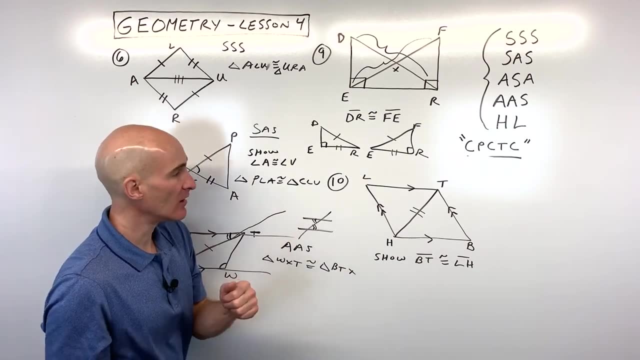 these single arrows and that's telling us that these lines, okay, are parallel, these opposite sides are parallel and, again, similar to what we did over here, okay, we use what we learned in a previous lesson about parallel lines and we can show that this angle and this angle are congruent. 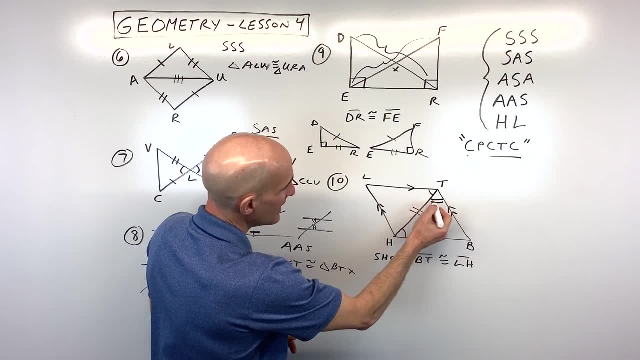 those are alternate interior angles. we can also show that this angle and this angle are congruent by alternate interior angles and if you have this on a sheet of paper, sometimes it helps to rotate the triangle. so we can show that this angle and this angle are congruent by alternate